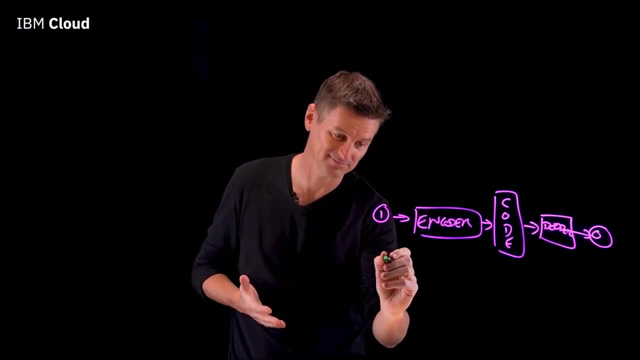 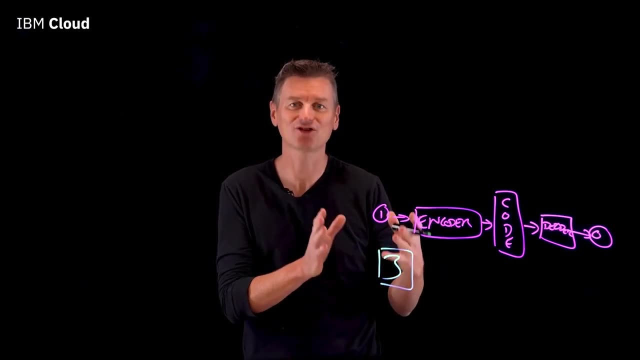 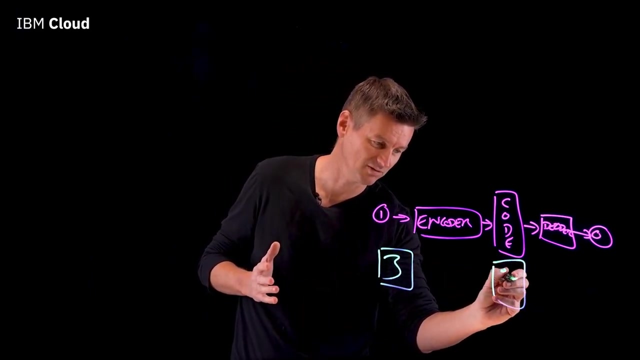 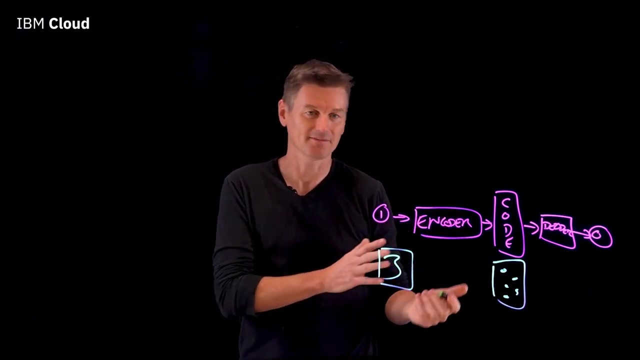 to images. So, for example, I can draw an image like this number three And then, through a process called feature extraction, I can derive the required features of the image by removing noise That looks a bit more like this, And then I'm able to generate an output that approximates. 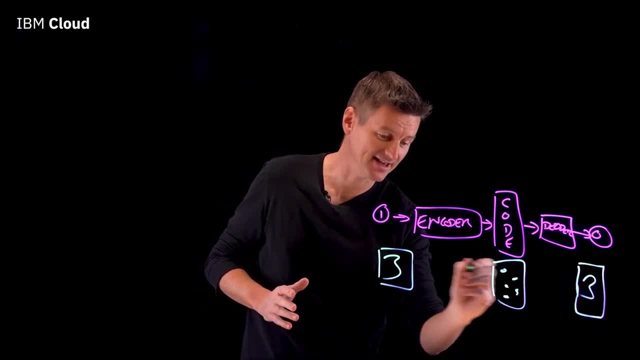 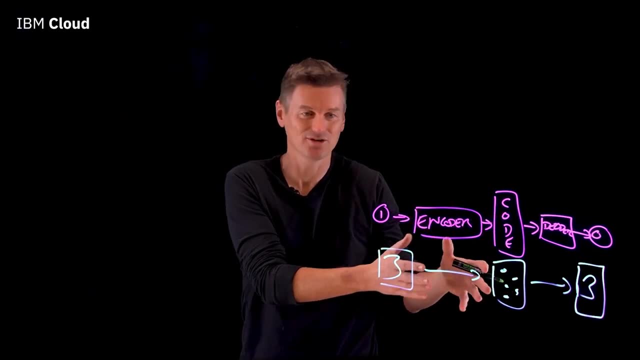 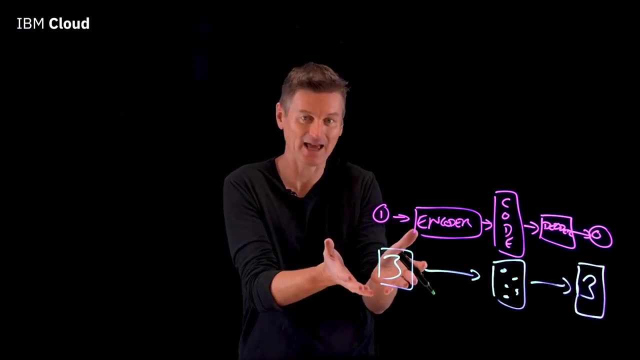 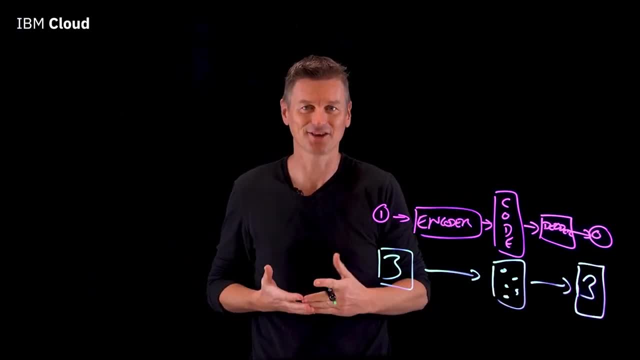 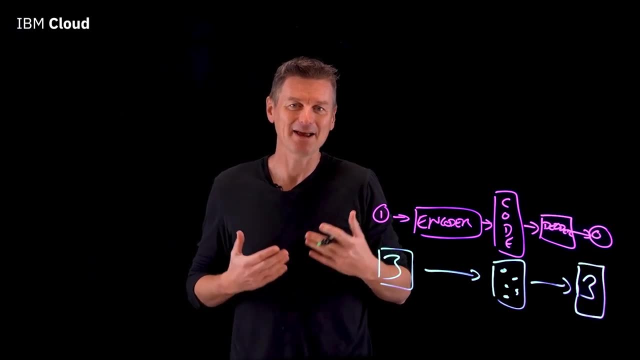 Now, in this case, the input and the output. they look much the same, which, well, that's what autoencoders are all about, but they don't have to be. We can provide input to an autoencoder in a corrupted form, like the noisy image of a 3,. 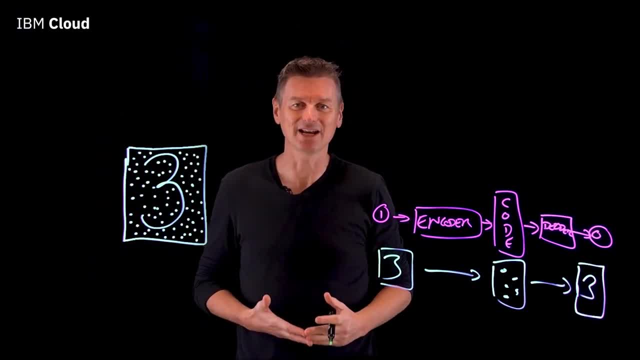 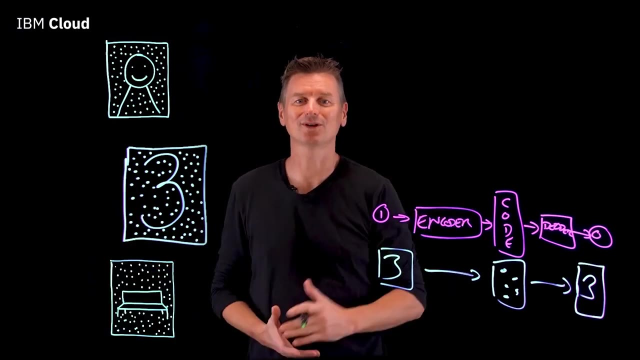 and then train a denoising autoencoder to reconstruct our original image from the noisy version of it. Once we've trained our autoencoder to remove noise from a representation of a number or a picture or a park bench, we can apply that to all sorts of objects. 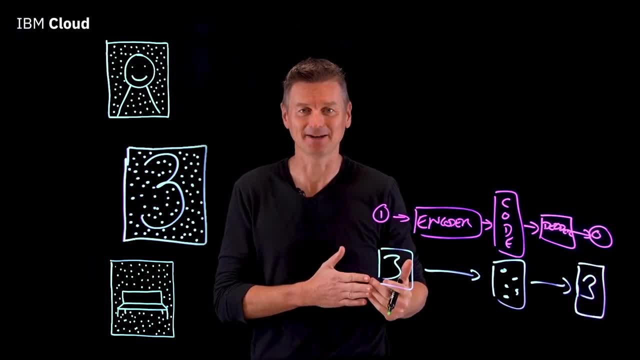 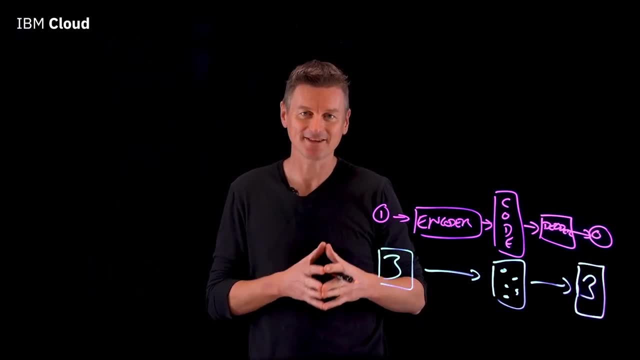 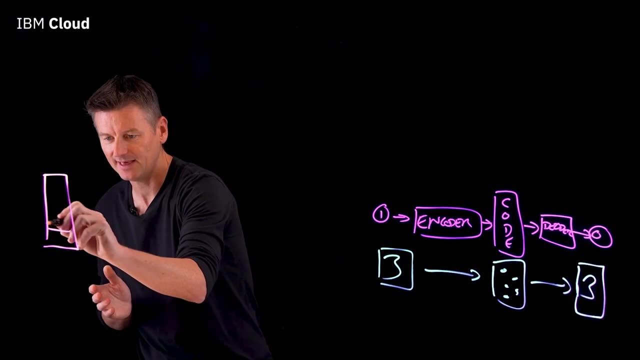 within an object element that displayed the same noise pattern. So let's take a closer look. inside an autoencoder, The encoder itself compresses the input into a latent space representation. So we have multiple layers here that represent the encoder. Each one 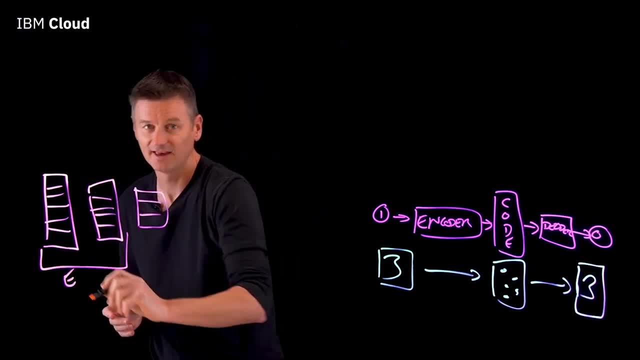 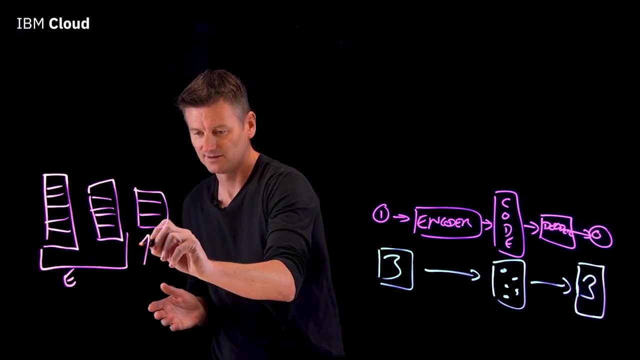 is a little smaller than the other. So this part here, that's the encoder, The most compressed version we said that's called the code. that's also known as the bottleneck, because I suppose much like the neck of a bottle.